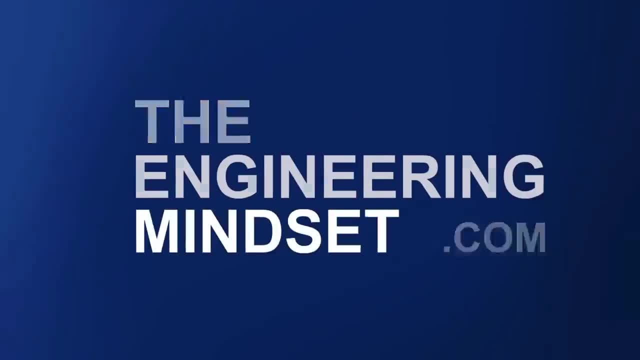 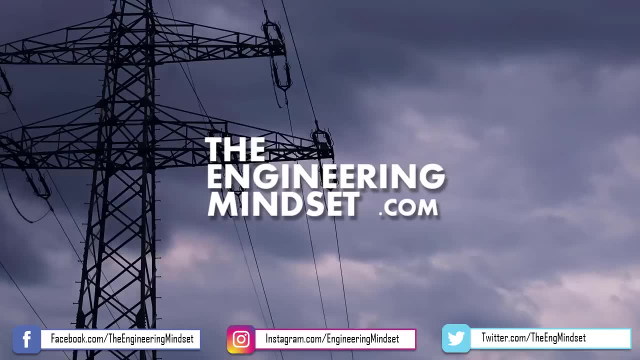 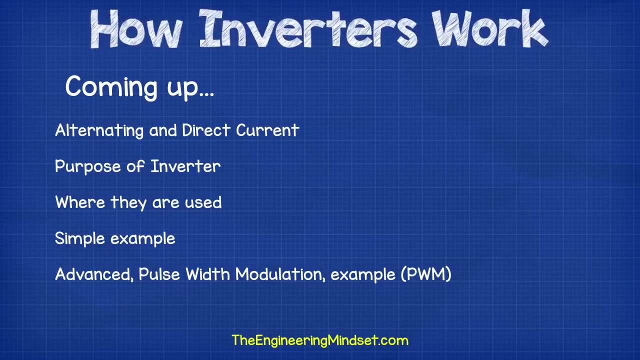 Hey there guys, Paul here from TheEngineeringMindsetcom. In this video we're going to be looking at inverters, their uses and how they work Coming up, we'll first of all look at the difference between alternating and direct current, then we'll look at the purpose of inverters and 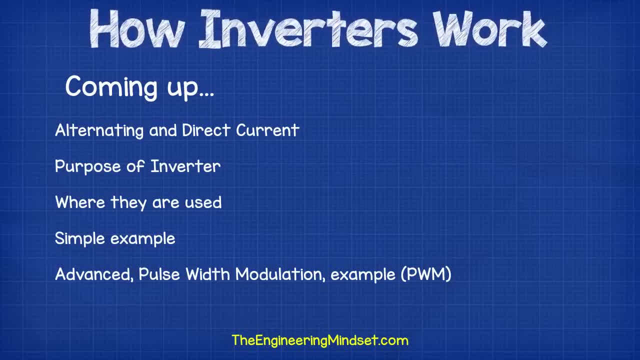 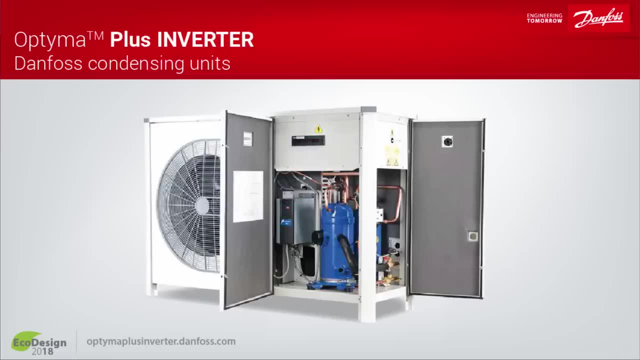 where they are used. then we'll move on and have a look at a simple example of how they work and finally we'll look at a more advanced pulse width modulation example. Guys, I just want to take a quick moment to thank Danfoss, our sponsor, for today's video. 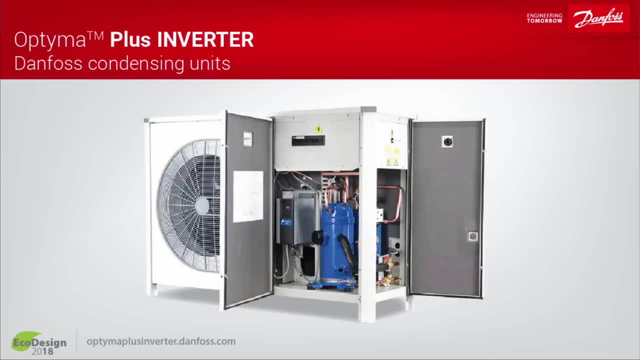 If you find inverters interesting, then you'll definitely want to check out the Danfoss Optima Plus Inverter Condensing Unit. The Optima Plus Inverter leverages stepless technology to increase efficiency and meet FGAS and EcoDesign requirements, and it's a great fit for applications in. 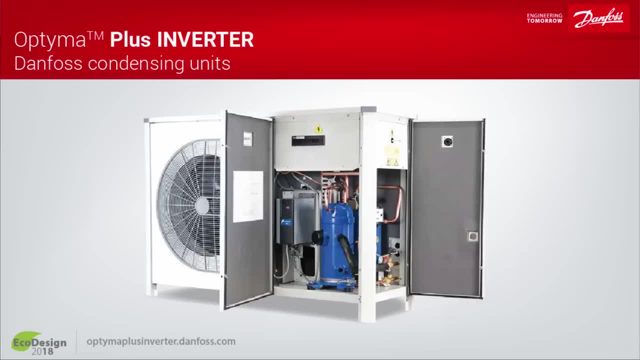 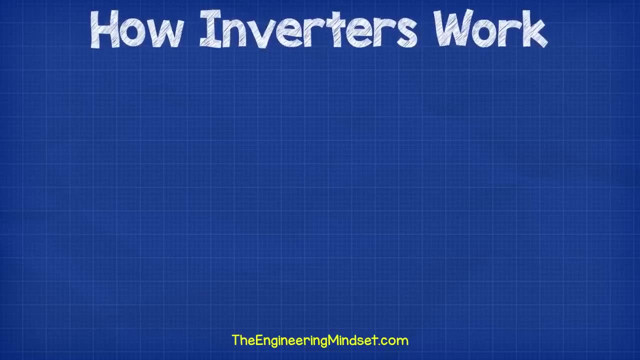 convenience stores and restaurants, etc. You can find out more about this great product at Optima Plus Invertercom. So what is an inverter? Well, let's start at the basics first of all. So you probably know that there are two types of electrical power in use, which are direct current or 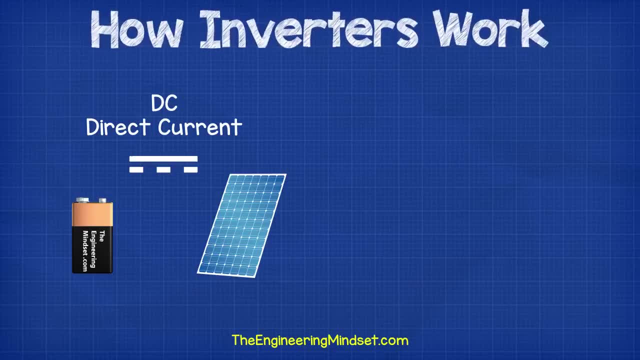 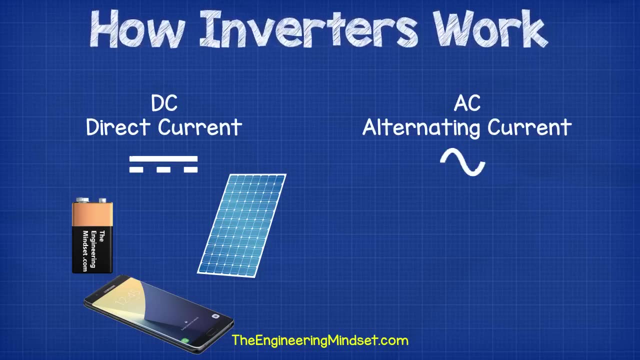 DC for short, which is supplied by batteries and solar panels etc. Now this type of power is mainly used by small digital goods with circuit boards etc. The other type of power is alternating current or AC. Now this is supplied from the power sockets in your homes. 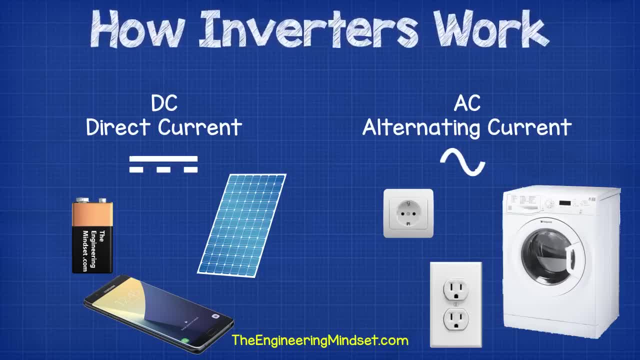 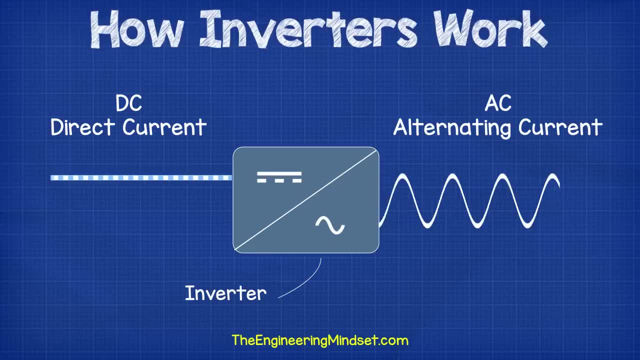 and this will typically be used to power larger appliances. Both of these types of power have their uses and limitations, so will often need to convert between the two to maximise their use. An inverter is a device which is used to convert between direct current and alternating current. 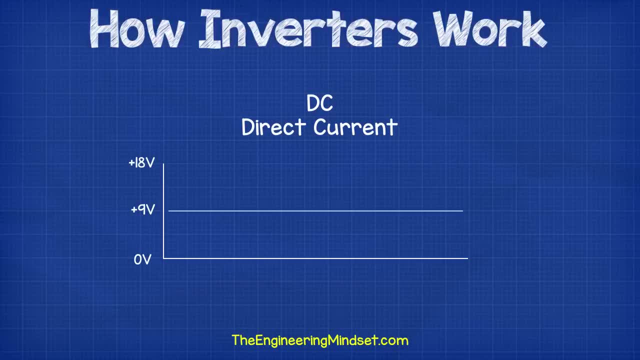 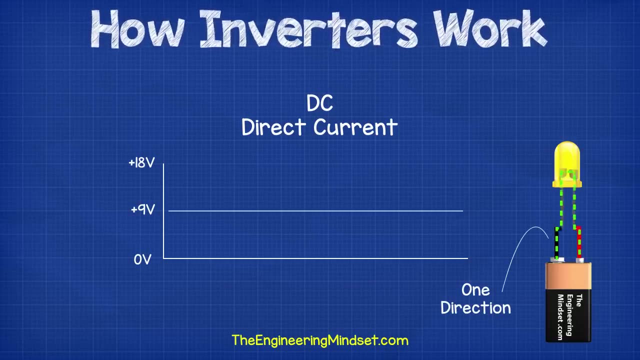 If you use an oscilloscope to look at the signal of these two types of power, you will see that direct current sits at its maximum voltage and continues in a straight line. That's because its current flows directly in only one direction, which is why it's called. 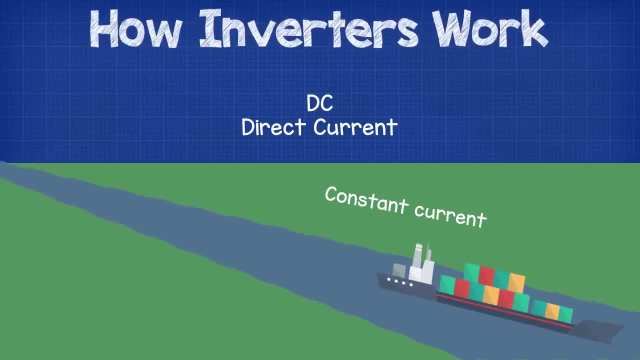 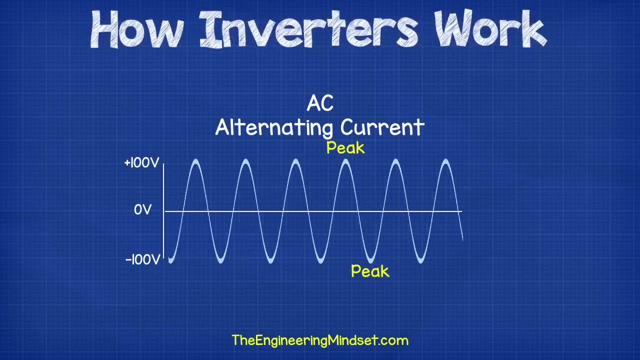 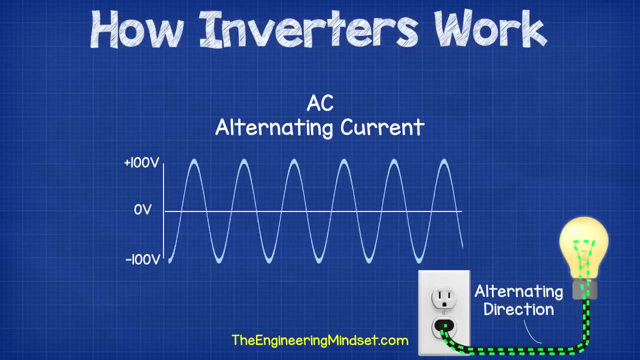 direct current. If you looked at alternating current, you'll see a wave-like pattern where the voltage alternates between its two peak voltages in both the positive half and then through to the negative half of its cycle. This is because the current travels back and forth. It's 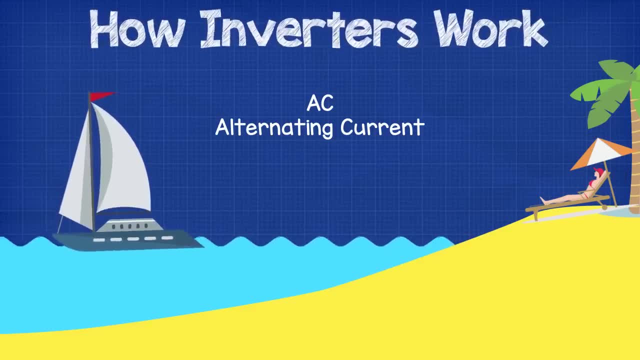 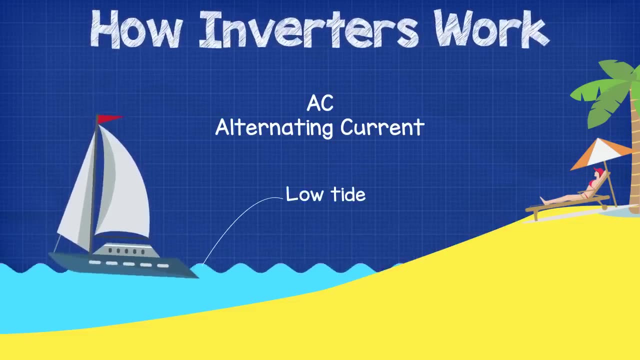 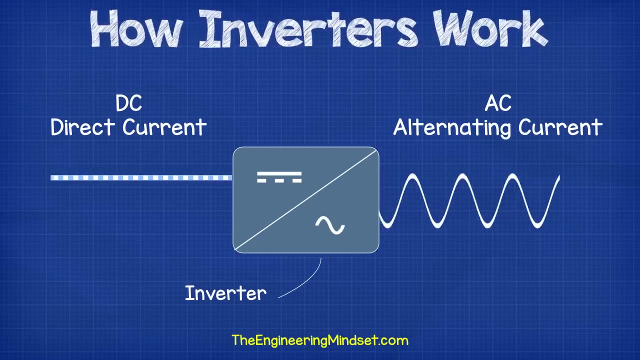 a bit like the tide of the ocean, where it reaches its maximum high tide and then transitions through to its maximum low tide, and in between the current of the seawater will flow and change direction. So an inverter simply converts from direct current to alternating current, and this 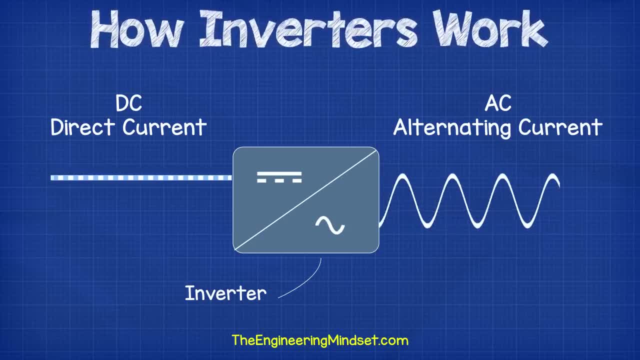 is a very useful invention. You can also convert from AC to DC using a rectifier, and it's common to find both of these in some devices. We'll actually look at this in just a moment. also, If you want to learn more on how electricity works, then start from the basics with our 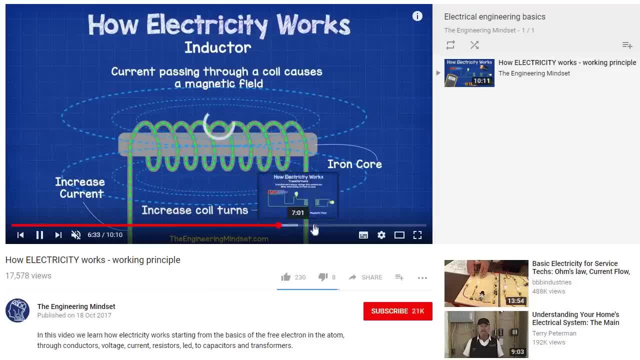 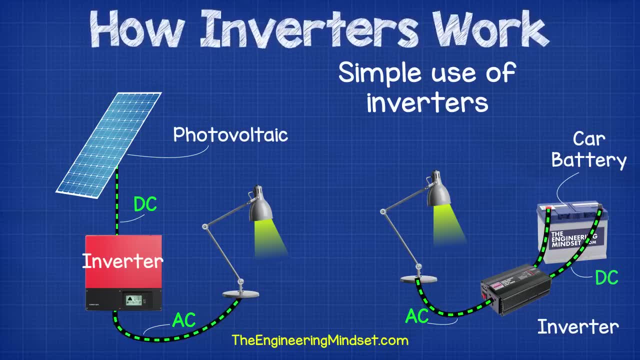 previous video on how electricity works. There's a link on screen now and there's also a link in the video description below. So where are inverters used? A fairly simple application of inverters is within solar panels or photovoltaic arrays, as these generate DC power, but the appliances in your home will use AC power, so this needs. 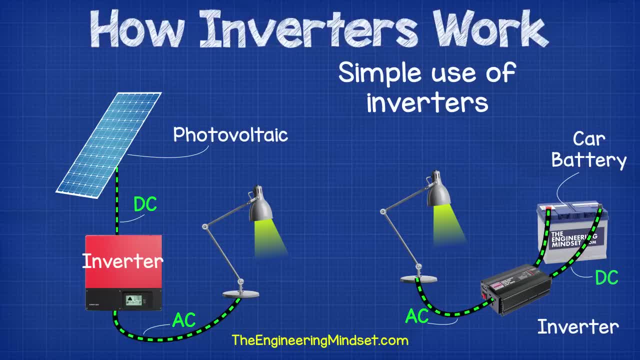 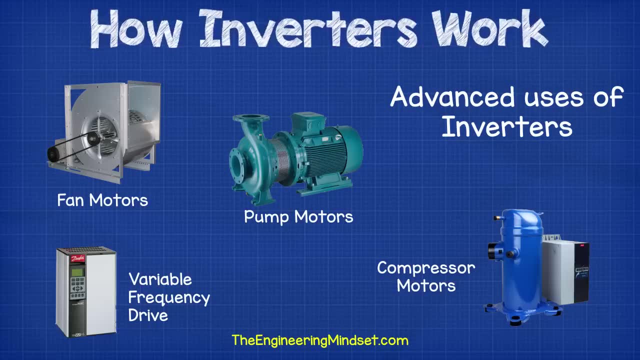 to be converted for it to be of any use. You can also buy portable inverters for your car which allow you to use the car's battery to power small household appliances. A slightly more complex way they are used is when integrated into variable frequency drives or variable speed drives to control the speed, the torque. 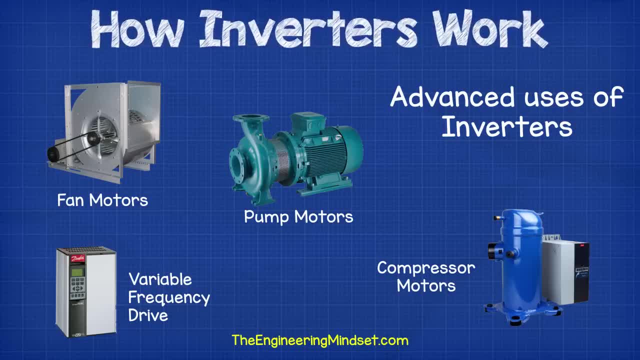 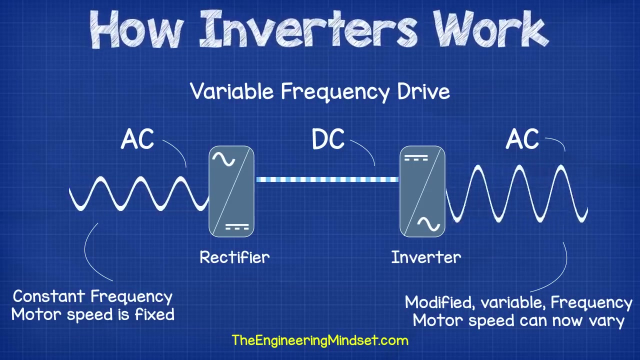 and the direction. In this application, the inverter is coupled with a rectifier and the AC power which comes in is converted to DC and then back to AC, but the controllers will change the frequency of the sine wave pattern. By manipulating this, we can precisely control how the motor behaves and when you join this. 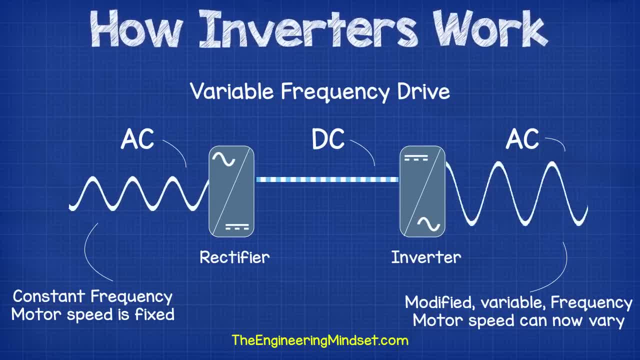 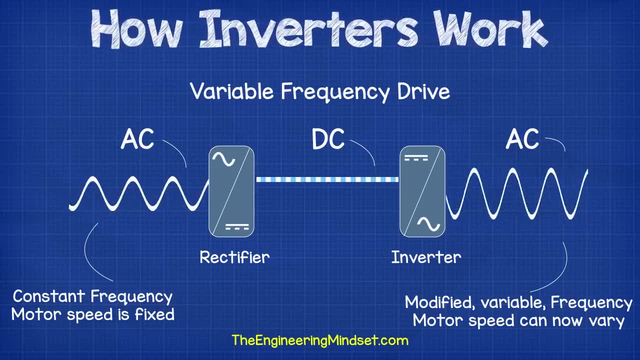 to a fan or a compressor etc. then you can precisely control how that performs. also, This is partly how the Danfoss Optima Plus inverter condensing unit works. It has a very clever control loop which is measuring the cooling load and then changes the speed of. 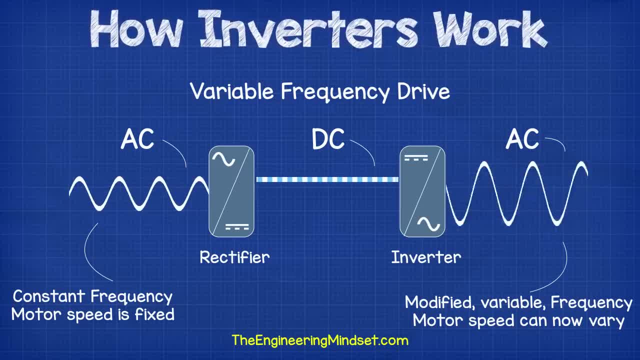 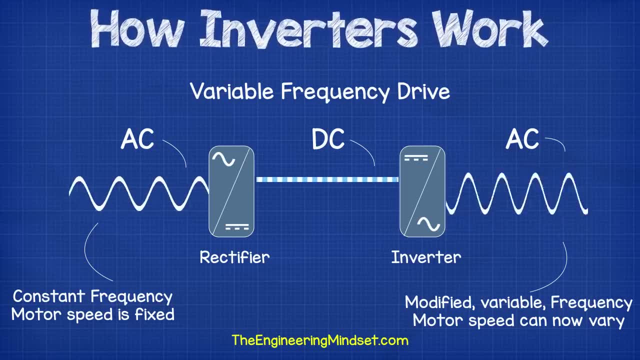 the motor which changes the speed of the scroll compressor and that increases or decreases the cooling capacity to match the load, which results in precisely controlling the cooling load, temperature control as well as energy savings. So how do they work? Well, let's consider a 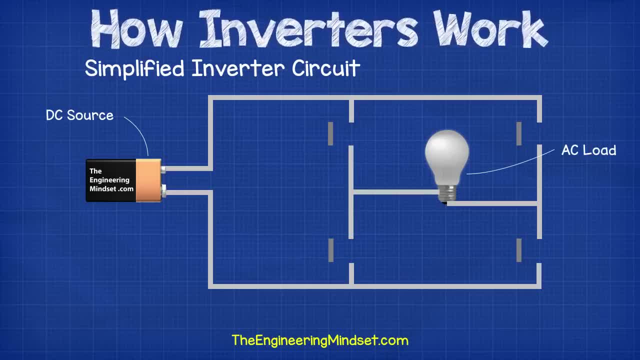 simplified circuit where the DC source is being used to power an AC load represented by the lamp. To convert the DC to AC, we will use four switches. We will pair the switches together so that switches two and three open when one and four close, and vice versa. This will allow us to force. 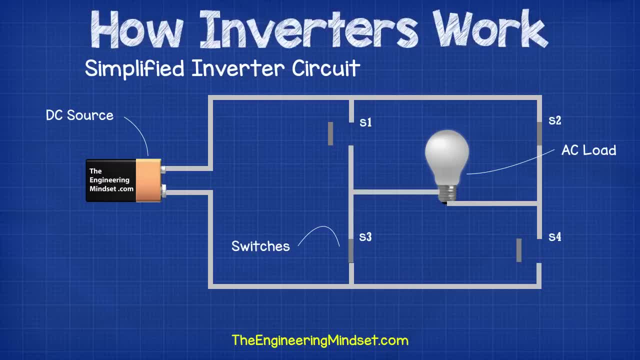 the current through the AC load in an alternating direction, so that the lamp will experience an alternating current, even though it's from a DC source. So let's give that a try. If we leave switches two and three closed and then open switches one and four, this will cause the current. 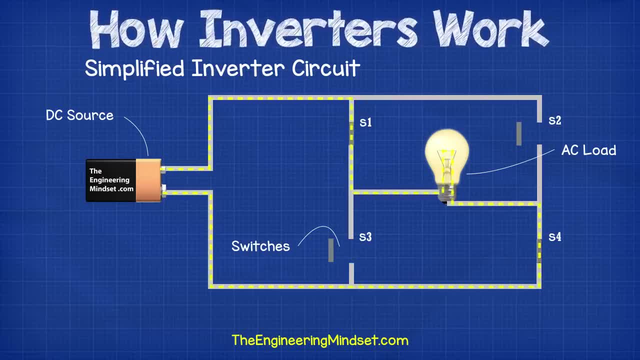 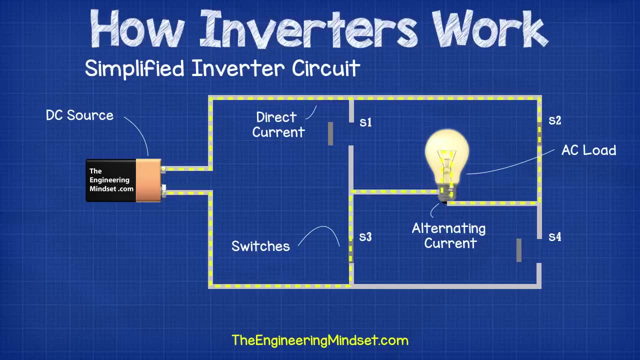 to flow through the right hand side of the lamp. If we then close switches one and four and open switches two and three, this will force the current to flow through the left hand side of the lamp. So you can see that there is a direct current source, but the lamp experiences an alternating. 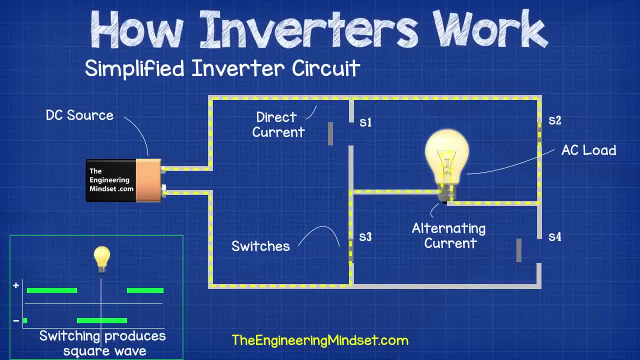 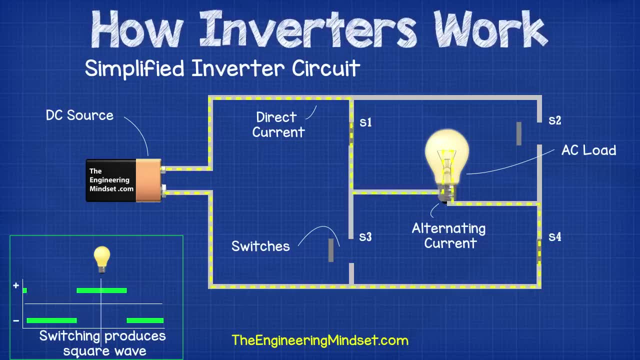 current. The lamp will not see this as a sine wave, However, as the sudden switching will only result in a square wave. The sharp corners of the square wave can be damaging to electrical equipment, so we need a way to smooth the corners out. The switching is also far too fast for a human to do, If you consider the electricity you receive. 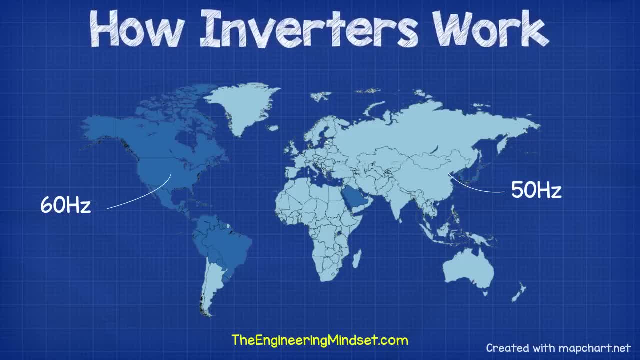 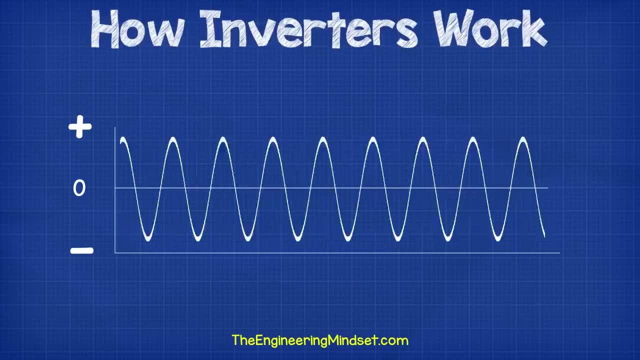 in the power sockets of your home. this will be supplied at 50 or 60 hertz, depending on where in the world you are. This means that the current needs to reverse direction 50 or 60 times per second. So to achieve this, we'll use some special electric current. We'll use some special 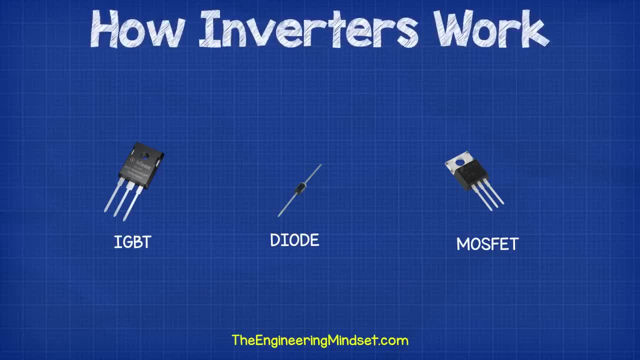 electronic components such as diodes, IGBTs, MOSFETs, etc. Now, if you don't know how these components work, don't worry about that for now. we'll cover this in another video specifically for that. For now, just understand the circuits and how the current is controlled. 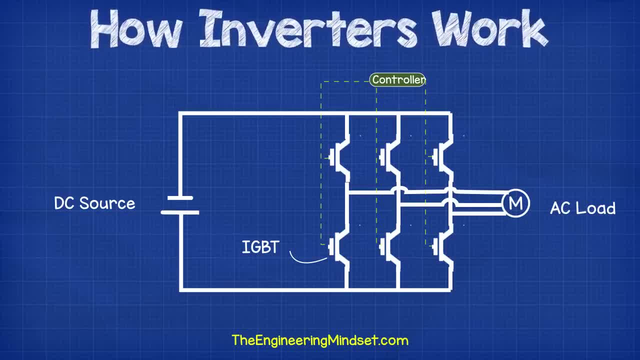 Let's look at a three-phase example for a motor. You can see this circuit has a DC source and an AC load and to convert the direct current into alternating current, there are a bunch of these IGBTs which are connected to a controller. The controller will send a signal to each IGBT, telling it when to open and close. 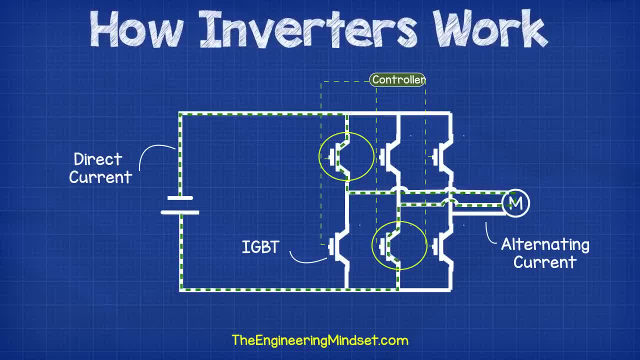 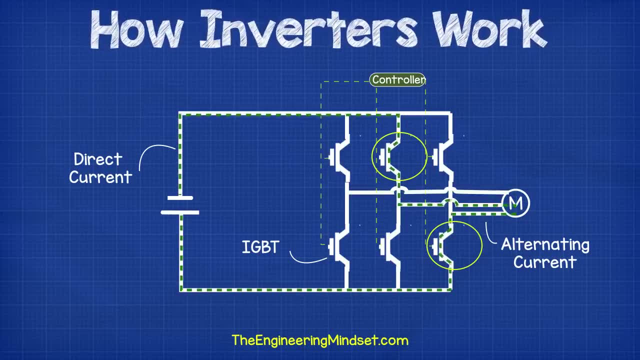 These IGBTs are paired together. So when the circuit is powered up, you can see that the controller is switching pairs of IGBTs to allow current to pass through them for a set amount of time so that the motor will experience an alternating current. In this example, the 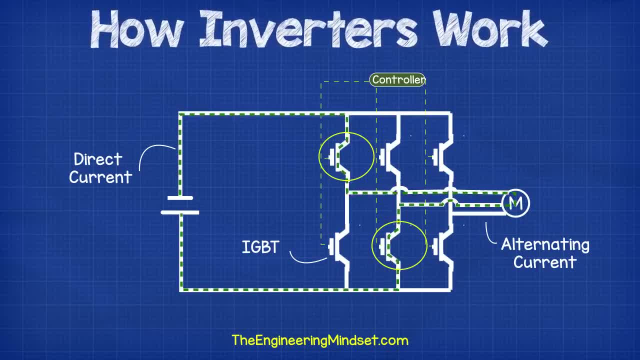 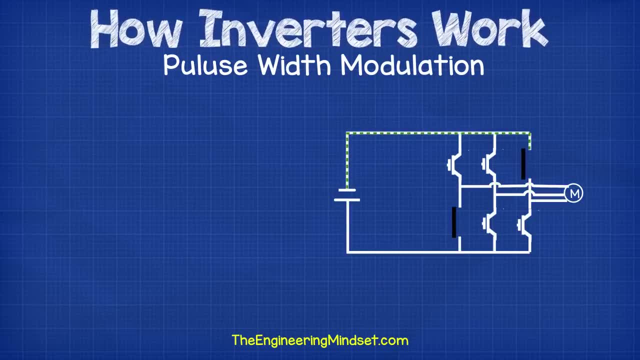 alternating current is in three phases, So this is used to power the motor, but how is it used to control the speed? Well, if we take a closer look at the IGBTs, we'll see that they actually open and close in a pulsating manner multiple times per cycle. This is known as pulse width. 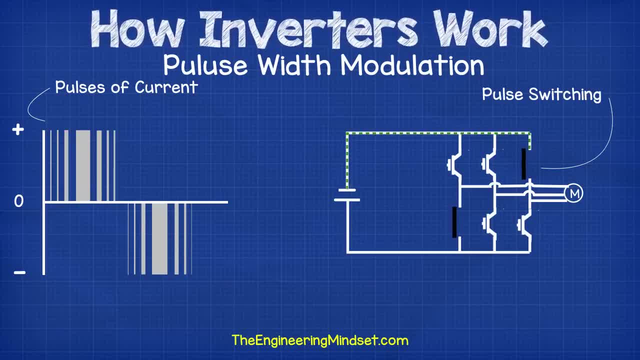 modulation. What's happening is the cycle has been broken up into multiple smaller segments and the controller tells the IGBTs how long to close for during each segment. I've shown how this works in just one cycle for one phase of the three-phase circuit, just to keep it as simple as. 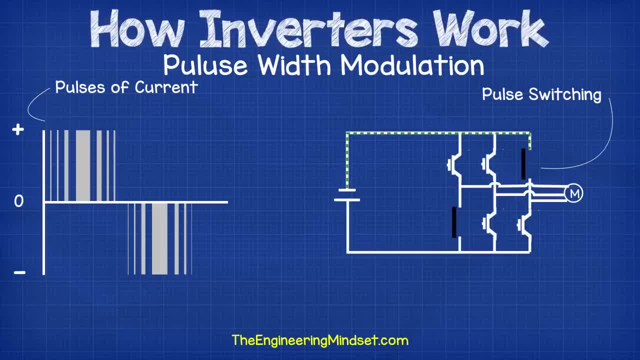 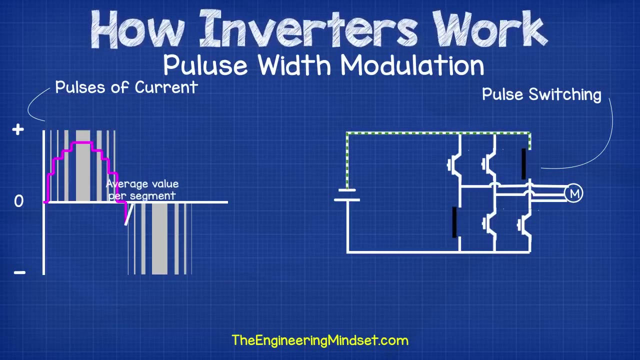 possible. By opening and closing the switches at varying lengths of time during each segment of each cycle. the IGBTs can allow varying amounts of current to flow through the circuit and into the motor. The result of this is that the average power over each segment will result in a sine wave pattern. The more segments 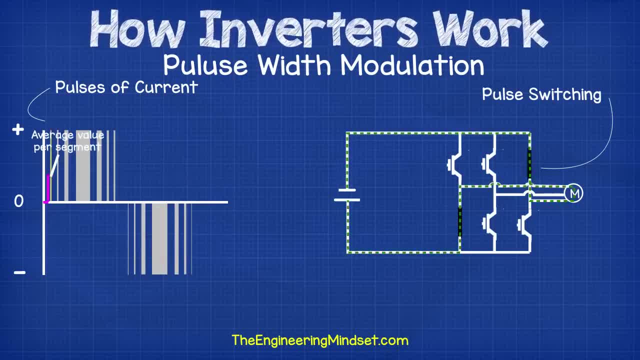 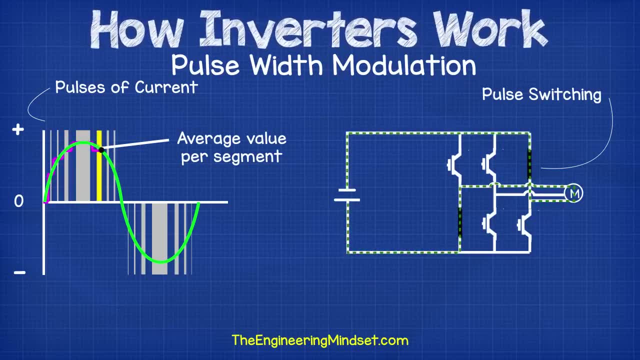 the cycle is broken into, the smoother the sine wave will be and the closer it will mimic a real AC sine wave. So the motor will see the average value and will therefore experience a sine wave alternating current. The controller can then change the amount of time the IGBTs are open. 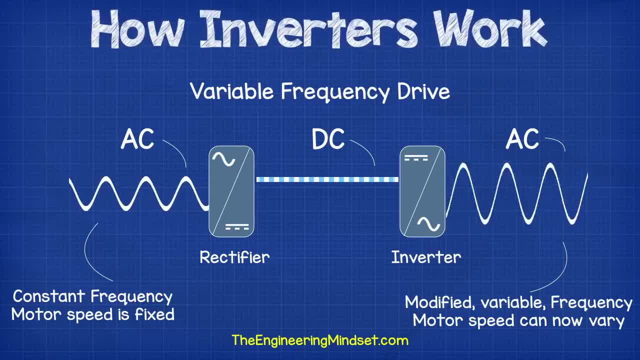 to increase or decrease the frequency of the IGBTs. The IGBTs can be used to control the frequency and the wavelength, to control the motor's speed, torque and direction, And with a few additional control loops it can be used to exactly match. 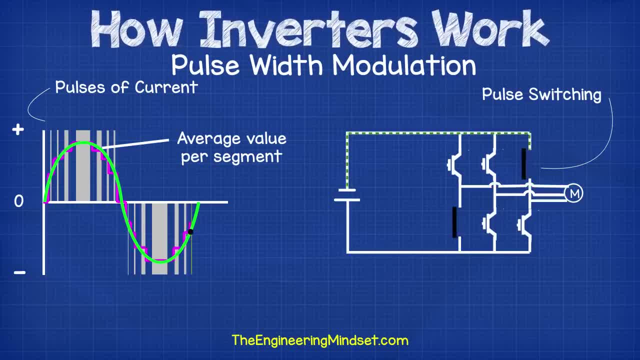 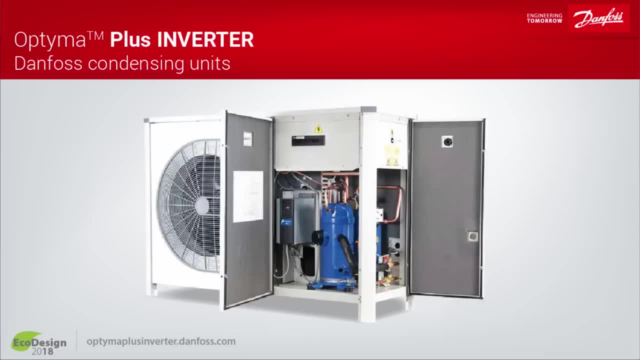 the required loading to provide precise control of a system and unlock energy savings. Okay, that's it for today. Before I go, I just want to thank Danfoss one last time for sponsoring this video. Don't forget to check out their Optima Plus inverters by heading over to. 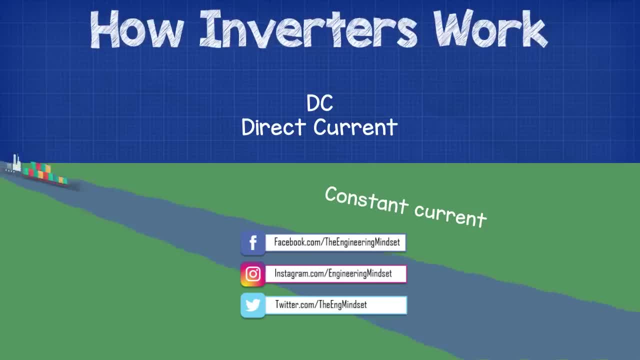 optimaplusinverterdanfosscom. Thanks for watching. I hope this has helped you and you've learned from it. If you have, then please like, subscribe and share. Don't forget to check out our Facebook, Twitter and Instagram, as well as our website, theengineeringmindsetcom. Once again, thanks for watching.